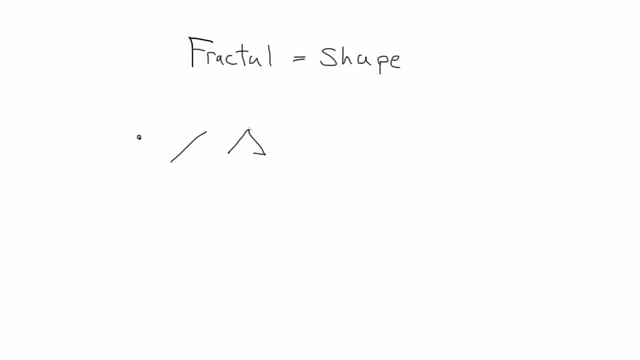 so it might be better to call it a pattern, but for our purposes a shape will do. Now, when you think of a shape, you might think of a point, a line, a triangle, a square, a circle, oval, or some kind of curve. Those are what I would call simple shapes. 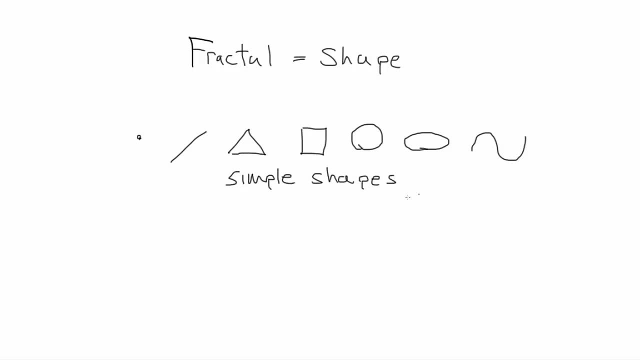 They're described with simple rules or a formula, and they simply are what they are. Then you have compound shapes like this house, for example. It's composed of two sub-shapes, a triangle and a square. Or this smiley face, which is a circle, a couple of ovals and a curve. 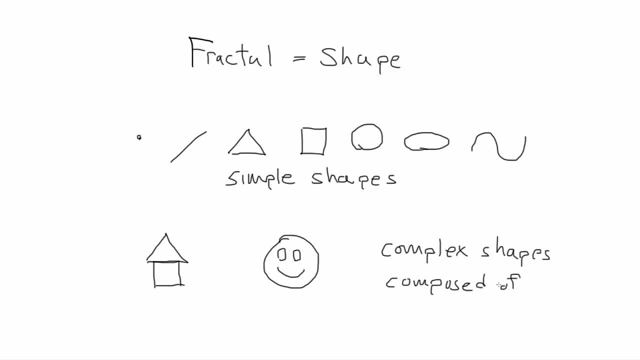 I'd call shapes like that complex or compound shapes, as they're made up of sub-shapes. A fractal is a special kind of complex shape where all of its sub-shapes are smaller copies of the shape as a whole. We call this self-similarity. You see, in some more advanced 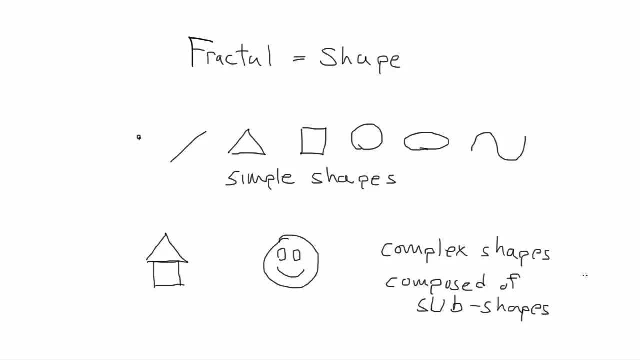 fractals, that the sub-shapes are more complex and the sub-shapes are more complex. Sub-shapes aren't always exact copies, but they are unmistakably similar. So say, we start with a triangle as our base shape. This means that this triangle should 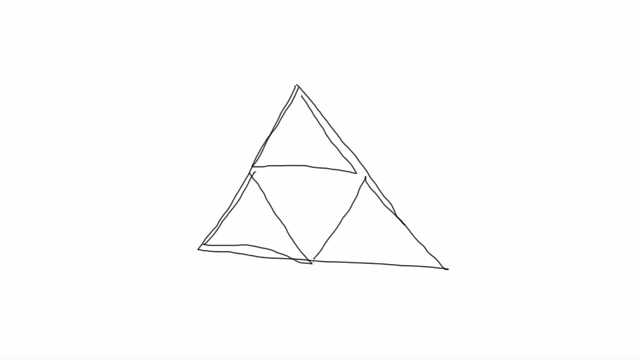 be composed of smaller triangles. So we do that. Now we have a triangle made of three triangles. Now some of you are saying that there's actually four triangles in there, and sure you could see it that way. But that center upside-down. 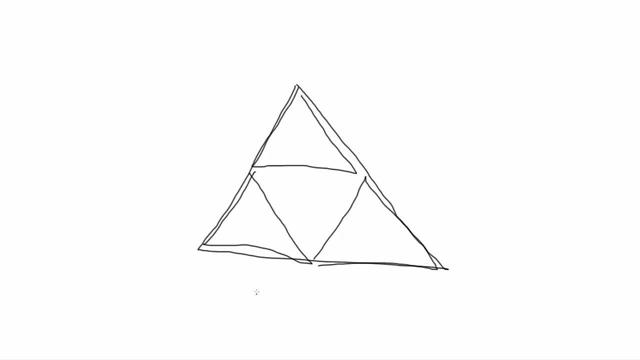 triangle is kind of a byproduct of drawing the other three, A triangle-shaped hole, if you will. So is that a fractal? Not quite, but it's a start. So here's our hole shape over here, a triangle composed of three triangles, And here is one. 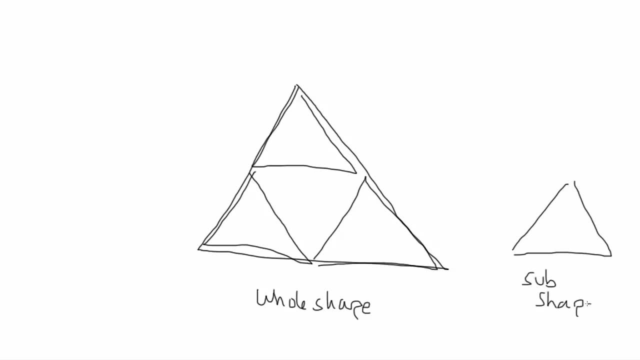 of those parts a simple triangle. Well, those aren't exactly the same, are they? The part should be a copy of the hole, so it should look like this, Which makes the overall shape look like this: Now, it's a triangle composed of nine triangles. 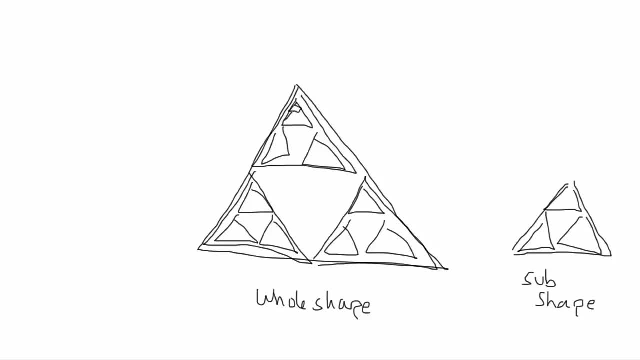 But the part is a triangle, made of only three triangles. So we subdivide the part again. but you see where this is going: Every time we subdivide the part, the hole shape gets more complex than each of its parts. The only way to solve. 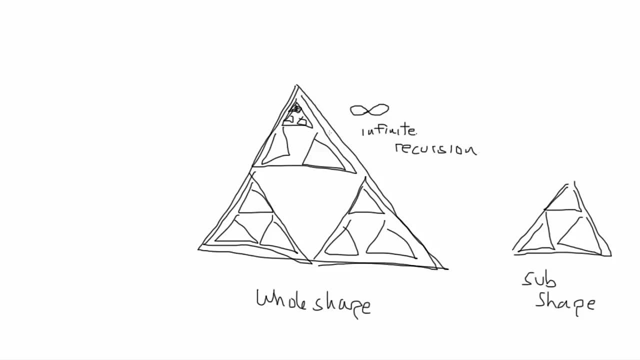 it is to iterate this infinitely, And that's another property of fractals. They're infinite, Or at least theoretically infinite, In the world of pixels or computer memory locations, or even atoms and molecules. eventually you get to a point where you just can't divide anymore. 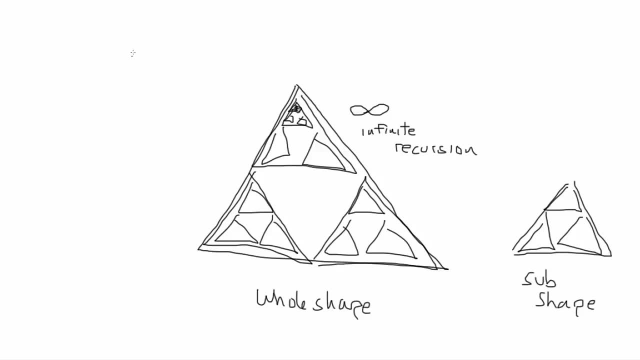 So in the world of pixels or computer memory locations, or even atoms and molecules, eventually you get to a point where you just can't divide anymore. But from a viewpoint of pure mathematics, yeah, they're infinite. Now, the name of this fractal shape, by the way, is the Sierpinski triangle, or Sierpinski. 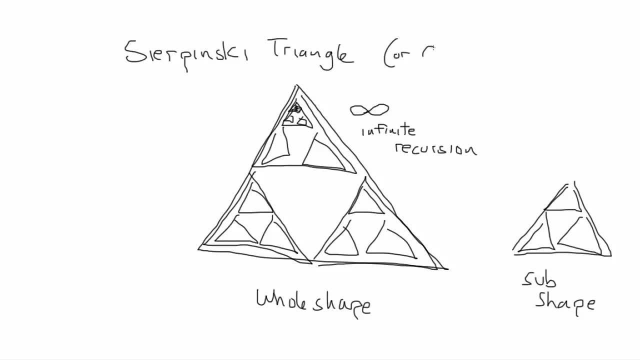 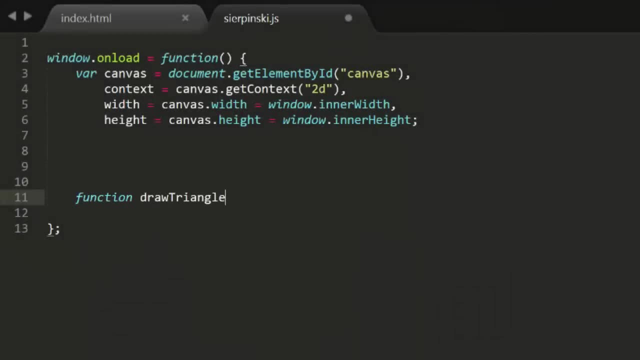 gasket. It crops up all over the place when you're making fractals. So let's see if we can code this thing up. Starting with the usual canvas template, I'll create a function called drawTriangle. It'll take three points. begin a path, move to the first point, line two to the next two. 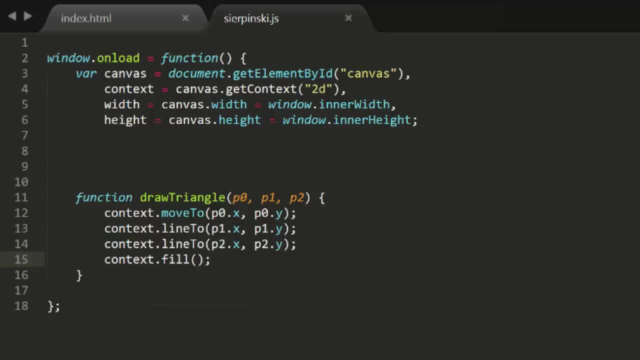 and fill, So we'll need three points to draw. I've pre-calculated a few points that will give us a roughly equilateral triangle. To start with, I'll translate the canvas so that its origin is in the center of the screen. 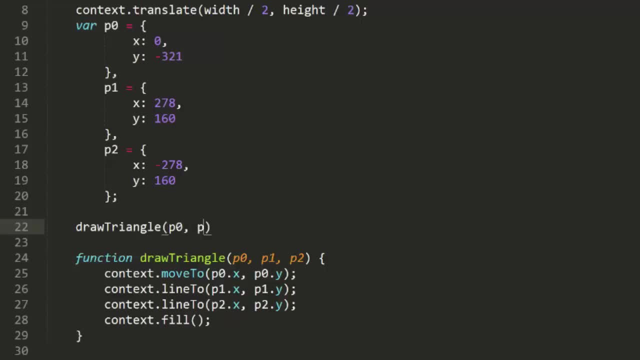 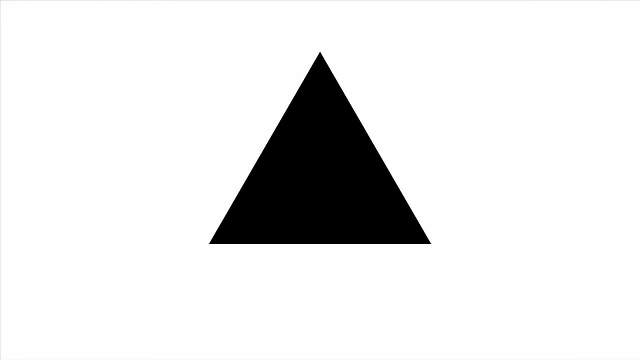 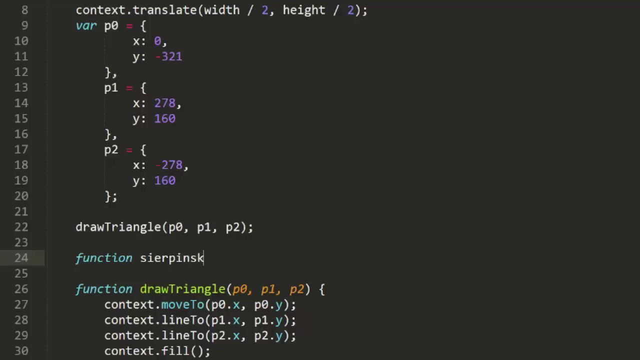 Then I'll paste in those magic points. Finally, we can call drawTriangle using those And run this, and we have a triangle. Now to fractalize it, I'll create a new function called Sierpinski. This too will take three points. 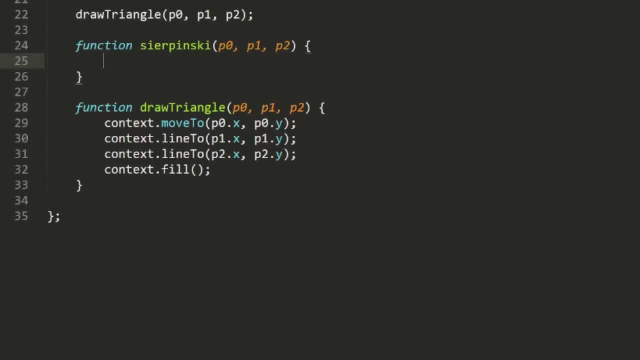 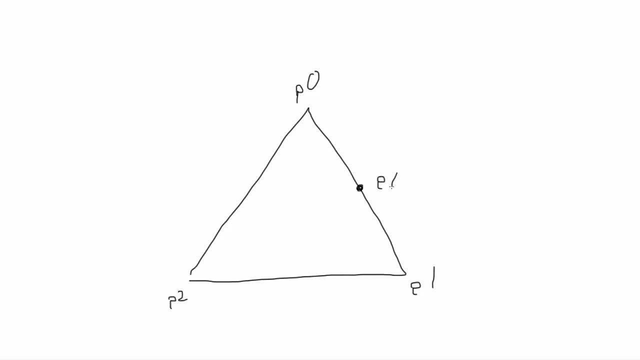 But it's going to calculate three more points right off the bat. Let me explain. We have our initial three points: P0,, P1, and P2.. And we're going to find the midpoint between each of the pairs of these points. 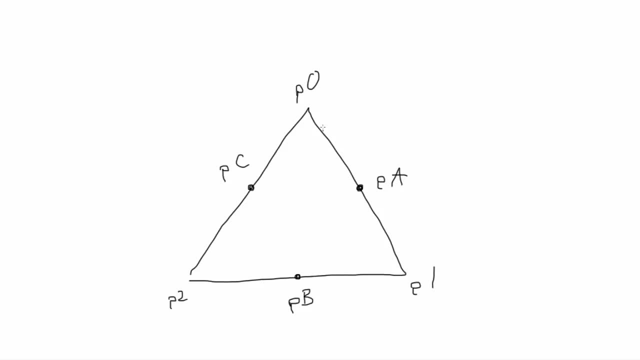 We'll call them PA, PB and PC. Then we can draw a triangle using PO, PA and PC, And another using PA, P1, and PB, And the final one using PC, PB and P2.. Let's do it in code. 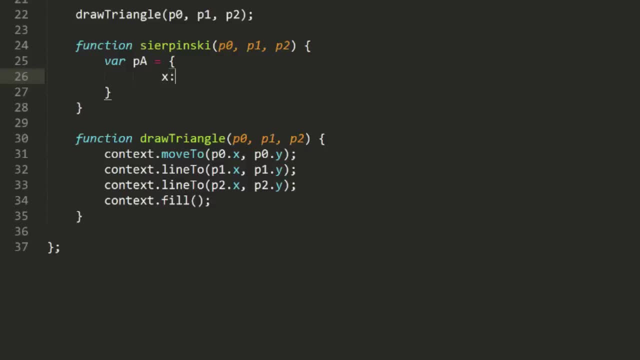 PA will be a point, with its x value equal to P0x plus P1x divided by 2. And its y value equal to P0y plus P1y divided by 2.. PB will do the same thing with P1 and 2.. 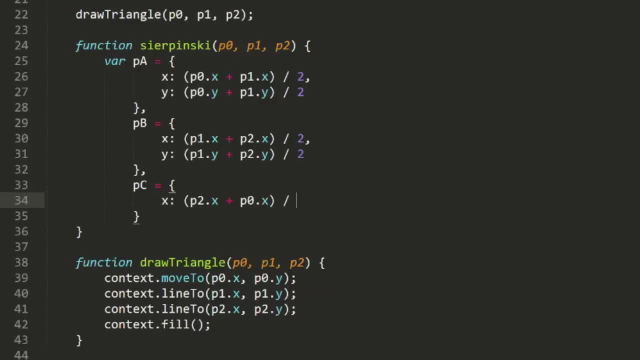 And PC will do the same thing with P1 and 2.. PC will be midway between P2 and P0. Now we can call drawTriangle using P0,, PA and PC, And again with PA, P1, and PB. 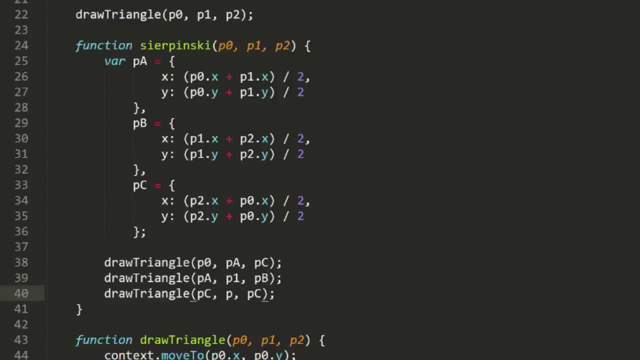 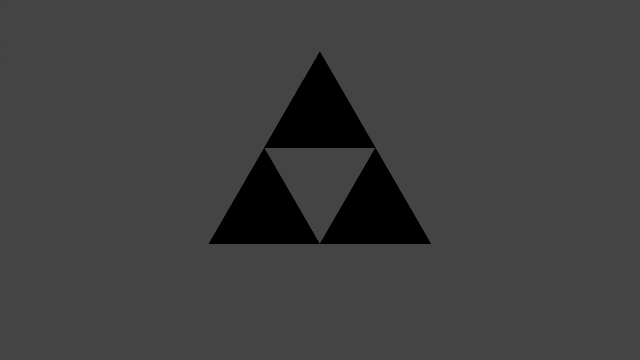 And finally with PC, PB and P2.. Then, instead of calling drawTriangle in here, we'll call syrpinski with those three initial points. Run it and we're one step closer to a fractal. Now we need to iterate each step. 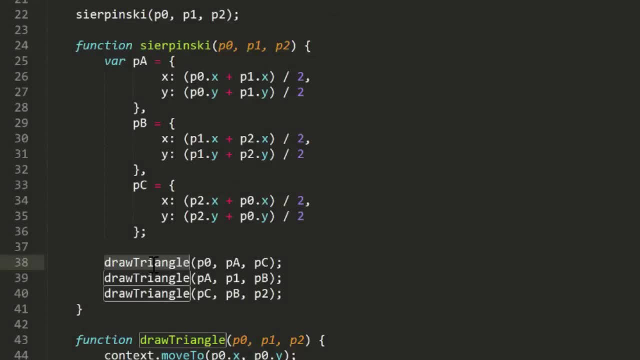 Instead of calling drawTriangle for each of those sub-triangles, we'll call syrpinski. We're moving into recursion, which is another common theme of fractals. This will subdivide each smaller triangle into three even smaller ones, and subdivide 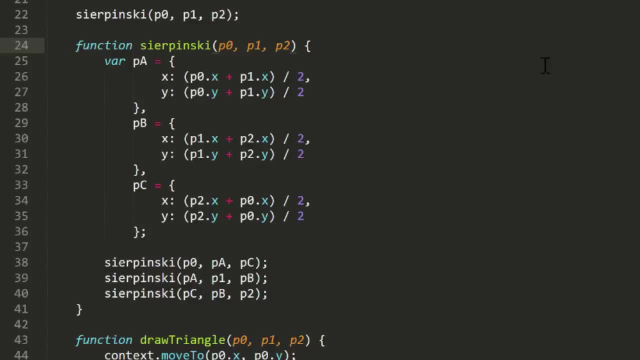 each one of those and subdivide those, etc. Of course, if we run this, it's going to crash or freeze up or do something really bad, Because computers don't like that. And even if the crashing weren't a problem, you'll see that we're never actually drawing. 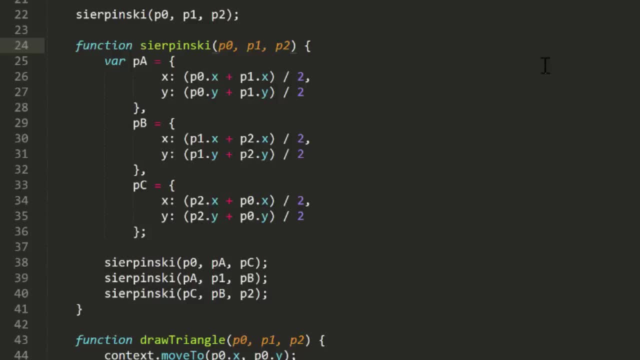 any triangles here, And even if we did, they'd be so small that you wouldn't be able to see them anyway. So we need to limit how many times we do this recursion. To do that, I'm going to add a fourth parameter to the syrpinski function, called limit. 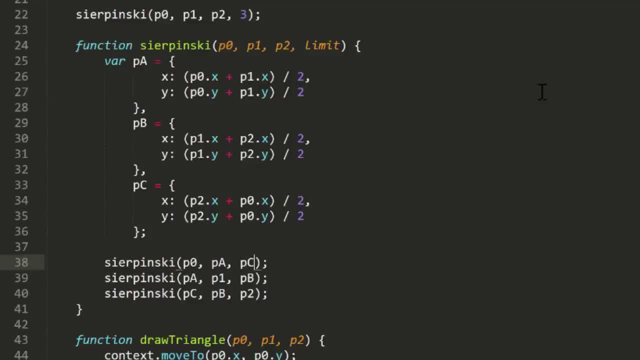 And I'm going to pass in a limit of 3 to the initial call. Now, within the syrpinski function in the recursion calls, we're going to add a limit of 3.. I'm going to pass limit minus 1.. 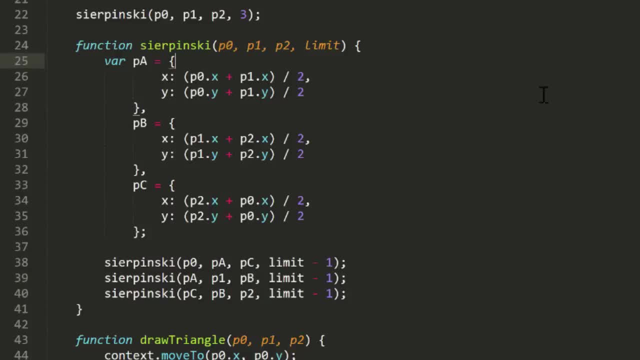 So, after a few iterations, limit will reach zero And we'll just use that as a flag to jump out of the recursive loop. I'll say if limit is greater than zero, and if so we'll just run the code that we've. 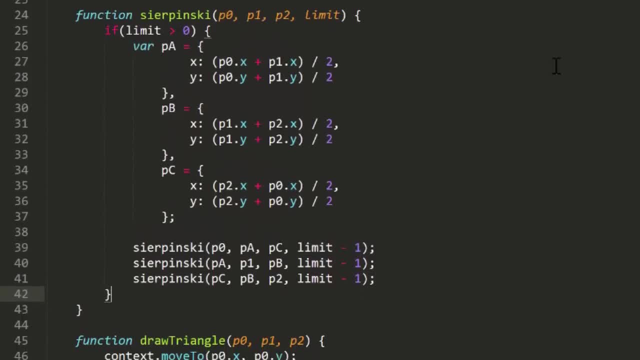 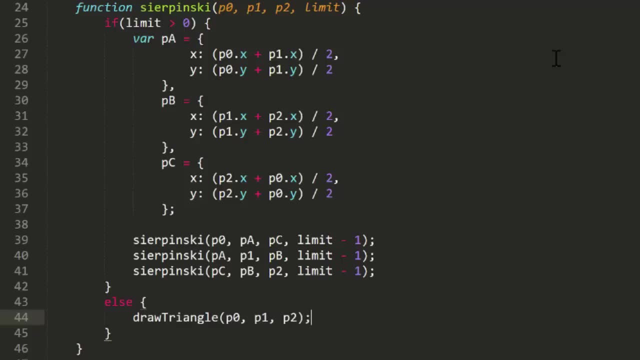 been running. But if limit reaches zero we'll go into an else block And there we'll just draw a triangle using the drawTriangle function. Now we can run this in C++ And we'll see what it looks like with three iterations. 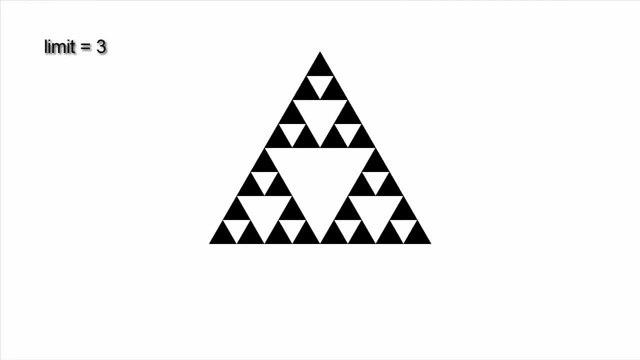 The triangles went from 1 to 3 in the first iteration, 3 to 9 in the second iteration and up to 27 in the third iteration. Here I'll change the limit to 4.. Then 5. And 6.. 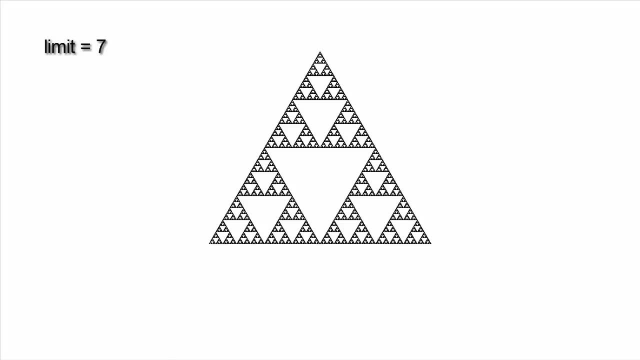 And when we hit 7, we're about at the limit of what's going to make a difference visually. Going to 8, and you're already below the pixel level and not a whole lot changes. Also, realize that the iteration is only going to be for the first iteration. 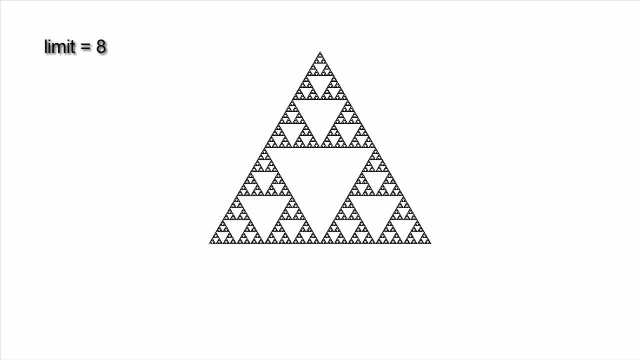 Also realize that at 8 levels of recursion we're drawing over 6500 triangles and you're going to start to see the program slow down as you multiply that number by 3 in each successive iteration. Realize that, although I pasted in points that made pretty close to an equilateral triangle, 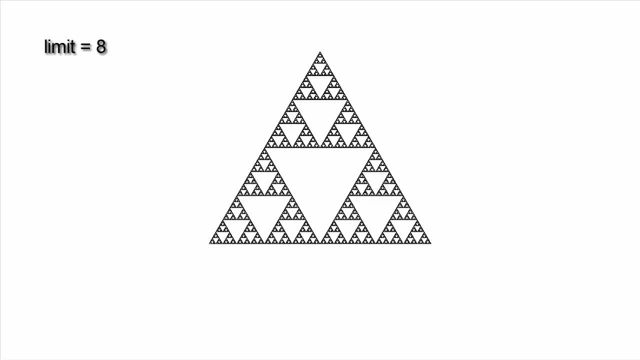 this will work with any triangle. Try messing around with the points or even randomizing them. What about another fractal? This is another famous fractal called the Koch curve. It starts with a series of 4 line segments all the same length. 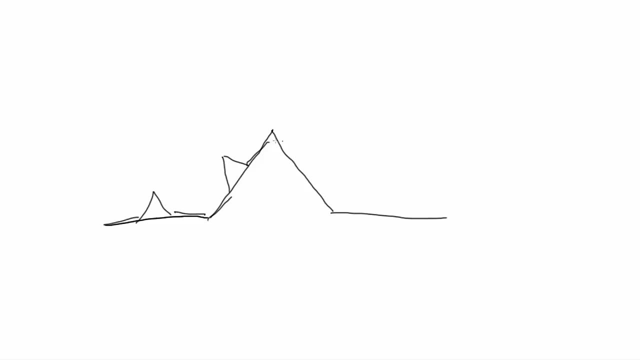 You then replace each of those line segments with the whole shape, like so: This gives you 16 smaller segments And you replace each one of those with the original shape And repeat to whatever level of infinity is practical To code this. we'll create a function called Koch that will initially just draw the curve. 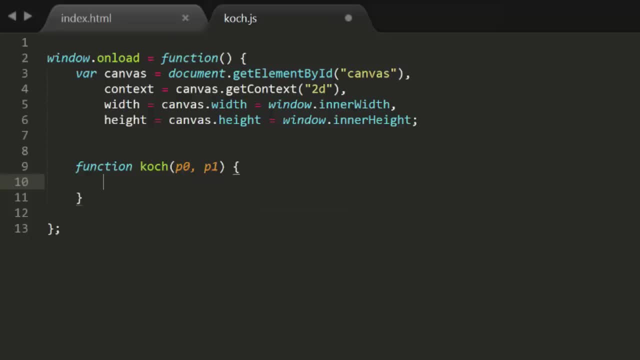 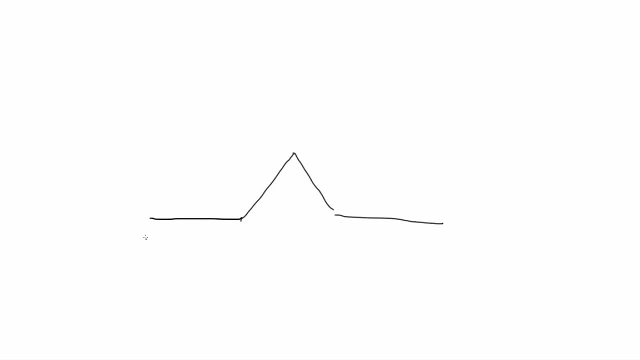 It will take two points: the start point and the end point. It will need to calculate 3 points in between those. Let's look at where those points need to be. Here's our start and end points. Call them P0 and P1.. 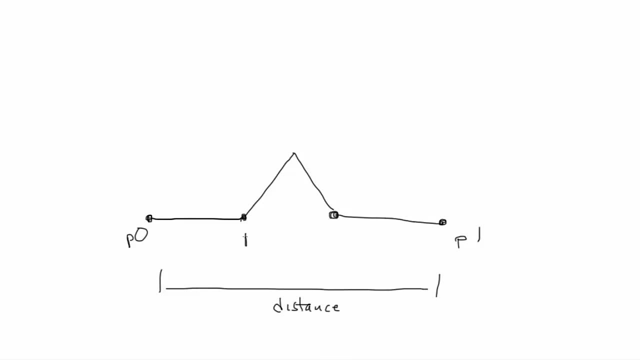 The first and last midpoints are easy. We just divide this distance into 3 parts. What we need to find is this point up here: The length of one segment will be 1 unit, So this point will be 1 unit away from this first midpoint, at an angle of minus 60 degrees. 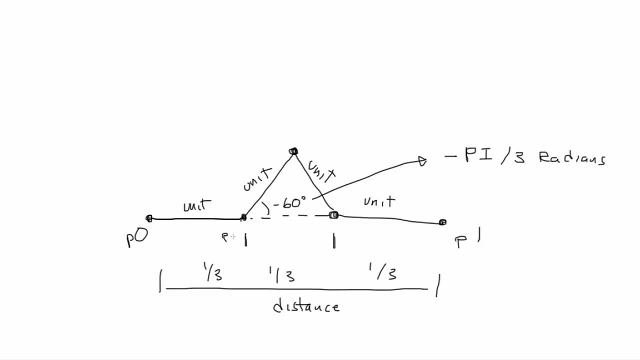 or minus 1.. Minus pi, divided by 3 radians. We'll call these midpoints PA, PB and PC, And we should be able to use some simple trig to find PB without too many problems. But first we should realize that P0 and P1 are not necessarily horizontal. 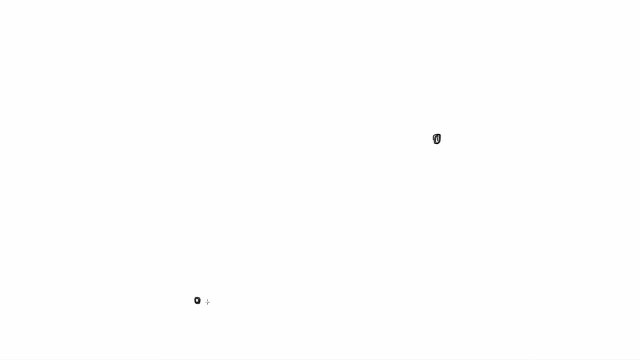 They could be more like this, And then we'd want to draw this curve like this. So we'll have to figure out this angle here and add that to the minus 60 first. Then we'll have the actual angle We need to find PB. 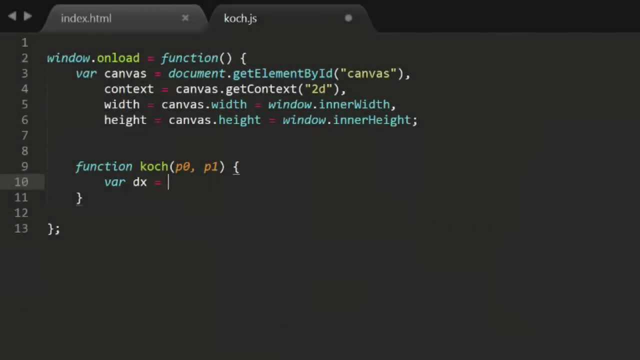 OK, back to the code. I'll get the distance between the two points on the x-axis and y-axis and then the total distance between them, And then I'll divide that by 3 to get the unit length of one segment. Finally, I can use mathatan2 with dy and dx to get the angle of the line between P0 and. 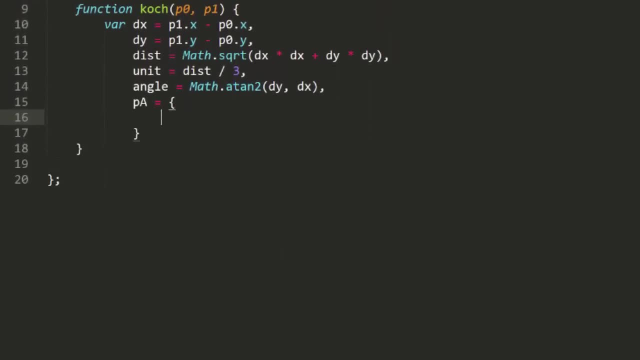 P1.. Now I can create point PA calculated by P0,, P1, and P2. And then I can use mathatan2 with dx to get the angle of the line between P1 and P2.. Likewise, PC. the last midpoint is simply P1 minus 1 third of dx and 1 third of dy. 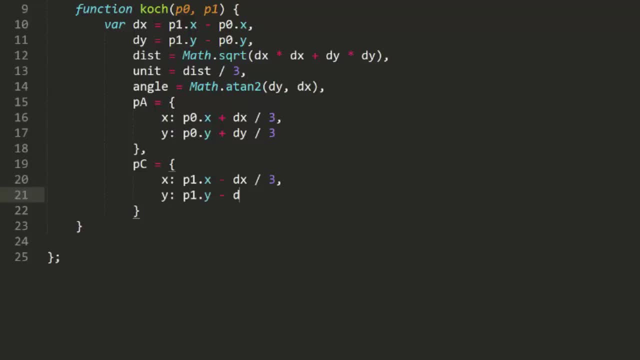 Finally, PB, the tricky one. Its x will be PAx plus the cosine of the angle minus mathpi divided by 3, times the unit length, And its y will be PAY plus the sine of that angle minus mathpi divided by 3, times that. 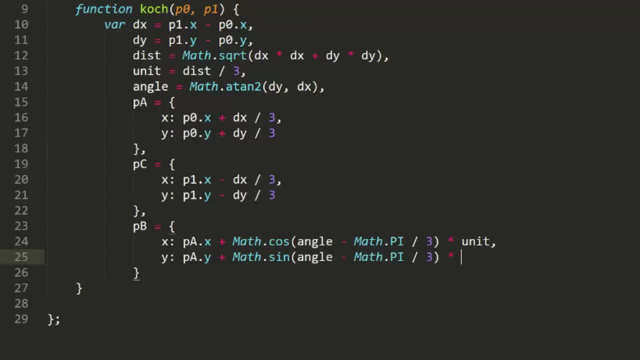 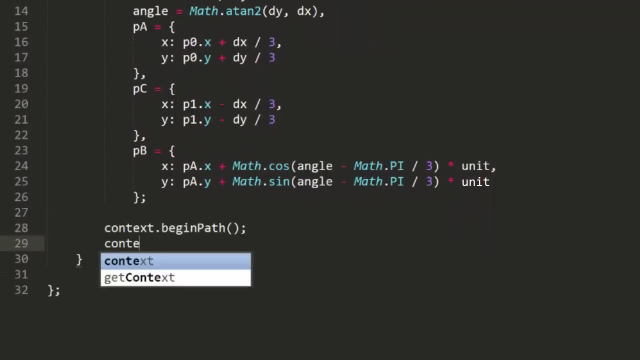 unit length. Refer back to that last drawing. if you don't totally get all that Now, we can draw the curve by moving to P0,, drawing lines to P A, B and C and finishing up with a line to P1.. 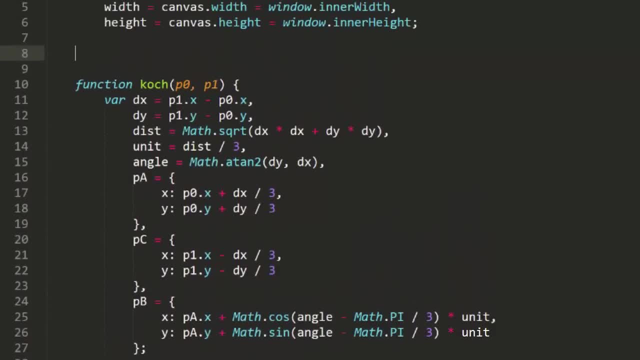 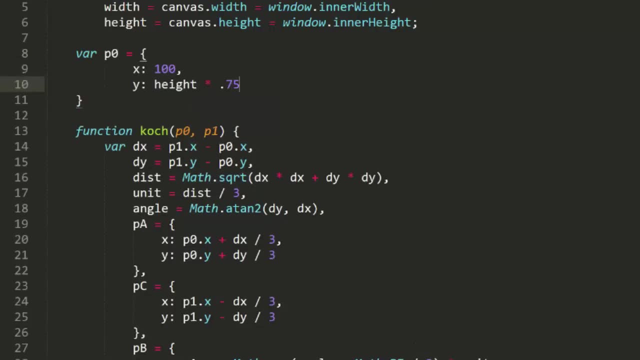 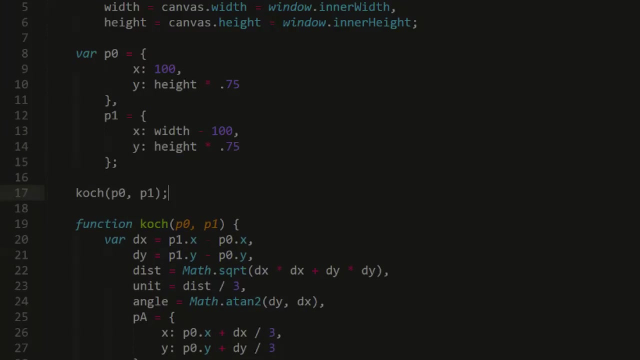 Finally, we just need to create the curve. OK, Let's iterate the two initial points and feed them to the function. First point will be on the lower part of the screen, on the left, and the other point, the same y, but on the right side of the screen. 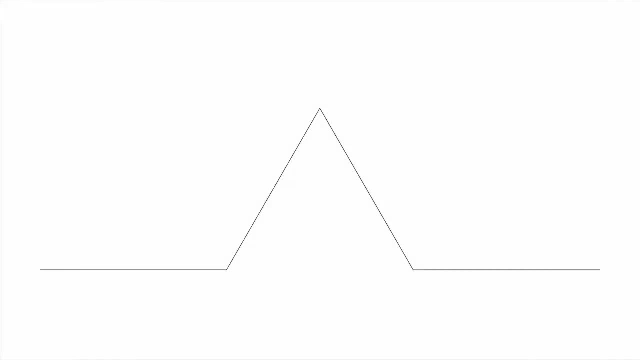 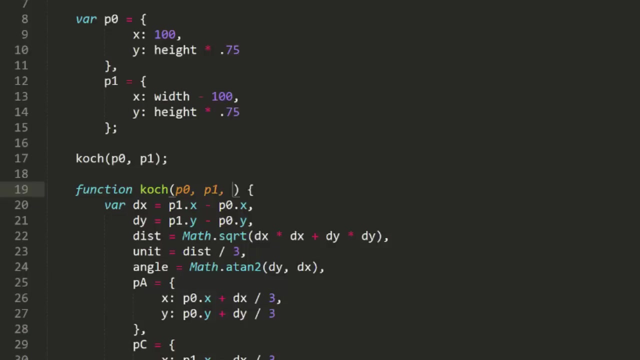 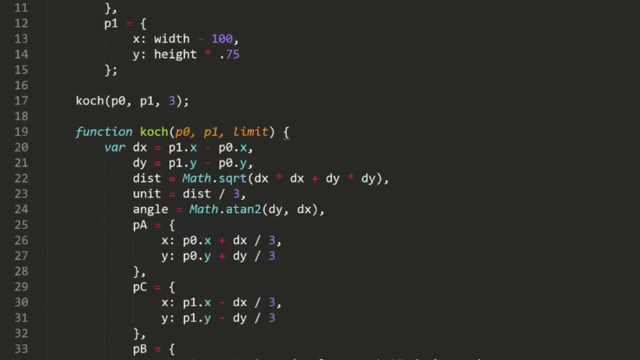 Test that and it looks good. Now we need to iterate it. We use the same strategy to limit the recursion, adding a limit parameter and making the initial call with a limit of 3.. We'll need those three points. we just calculated whether we iterate or not. 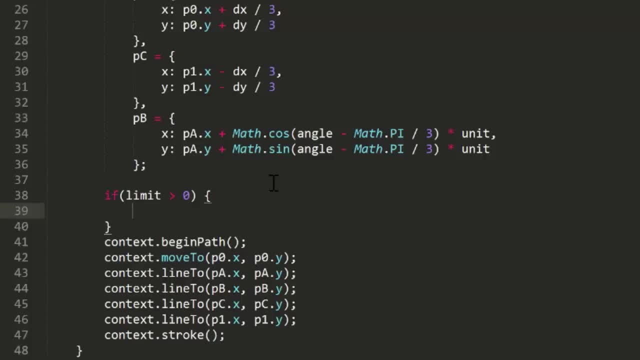 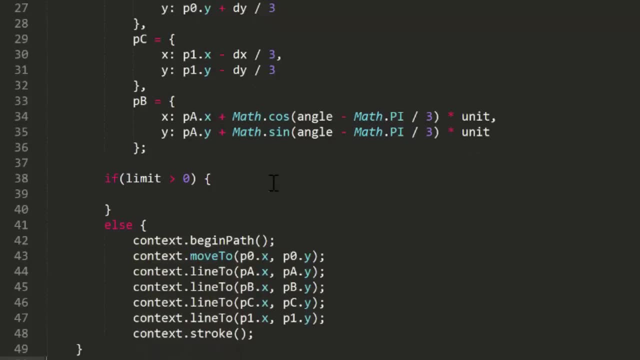 So after we create them we'll check if the limit is greater than 0.. If so, we'll leave an empty block for now And in the else block we'll draw the lines. Now we can do the iteration in that first, if block. 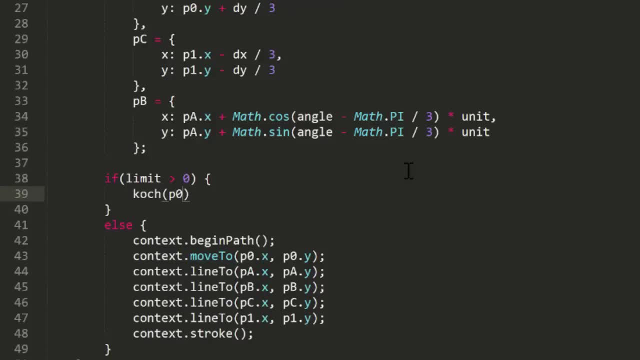 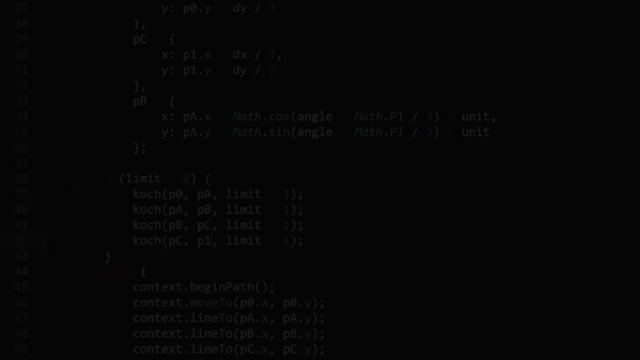 We simply call the Koch function, again with P0 and PA and limit minus 1.. And then the same for PA and P0. And we're done OK. And then for PB and PC And finally PC and P1.. 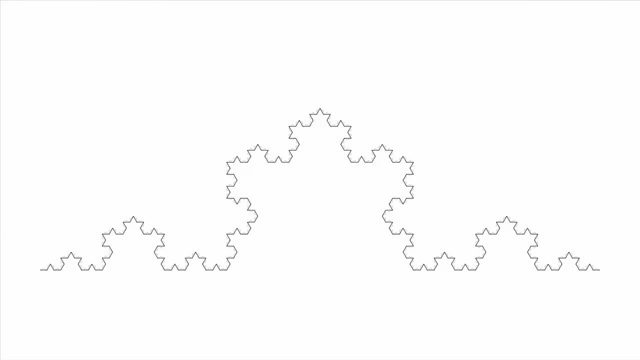 We run that and we have three iterations of the Koch curve. Crank up the iterations a bit and we can see where it leads. Same concepts about limits apply as before. More iterations mean more and more line segments. Eventually you'll have a whole lot of them and they'll be too small to notice any difference. 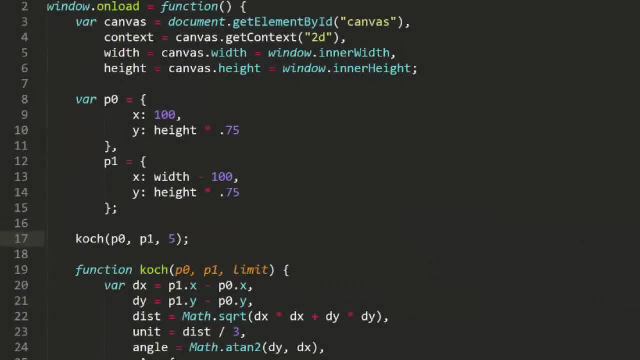 between iterations. Now, a variation on this is to take the same three points we used for the Sierpinski triangle and copy them in here, And because those points were based on translating the canvas to the center screen, we'll do that as well. 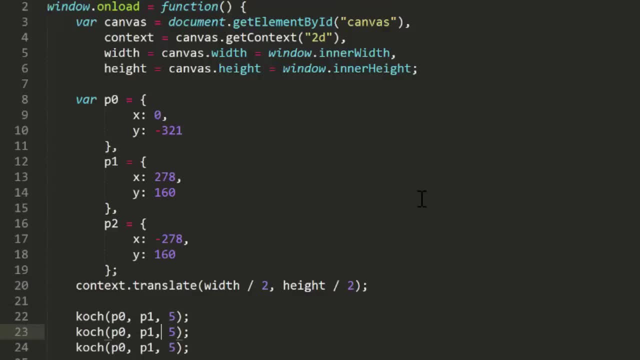 Then we can draw three Koch curves: from P0 to P1, P1 to P2, and P2 back to P0.. This is called the Koch snowflake. Now let's take a look at the Koch curve. This is called the Koch snowflake. 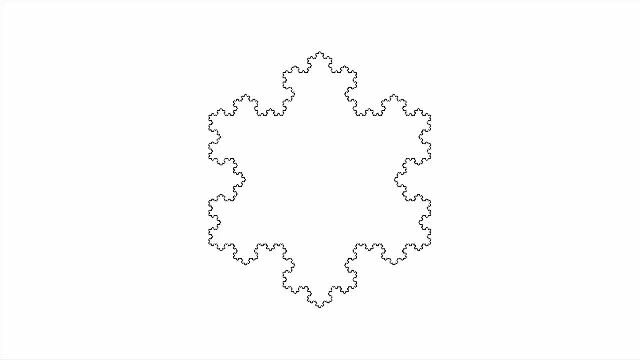 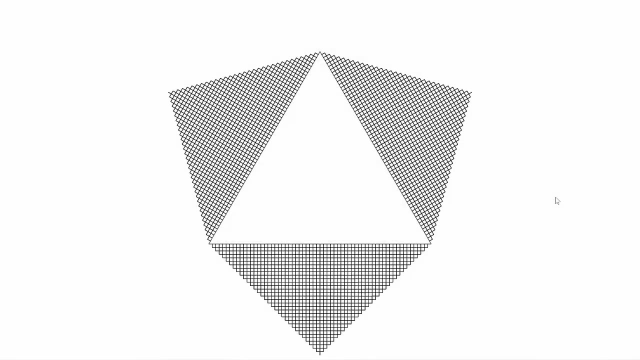 So there you go with a couple of simple fractals. Don't stop here with them. Although I've coded both of these up countless different times, I always find something new to do with them. While I was writing the code for this episode, I started messing around with some of the 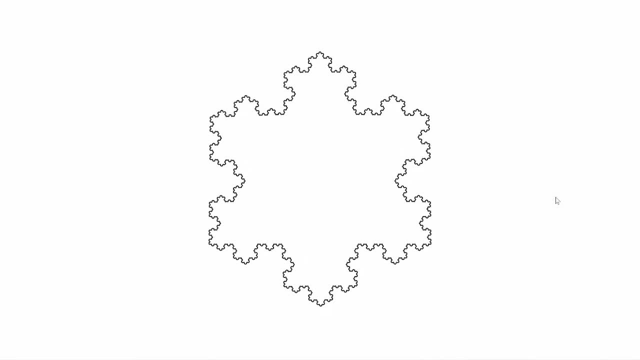 parameters for the Koch code and animating it, And I came up with this. I thought that was pretty neat And when I was fooling around doing the same thing with the Sierpinski code I got this Kinda blew my mind. 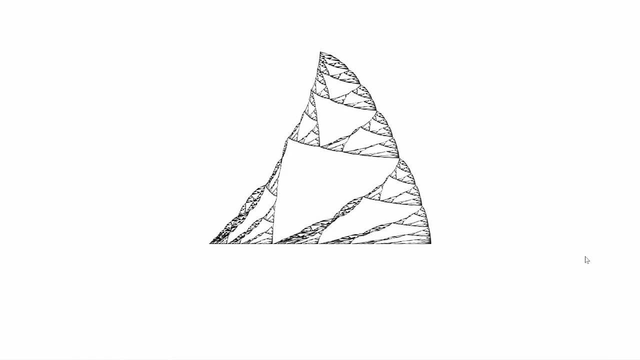 I'll put the code for these in the GitHub repo too. Play with it, Put it back together again, Wrong, And see what happens Above all have fun. Thanks for watching.